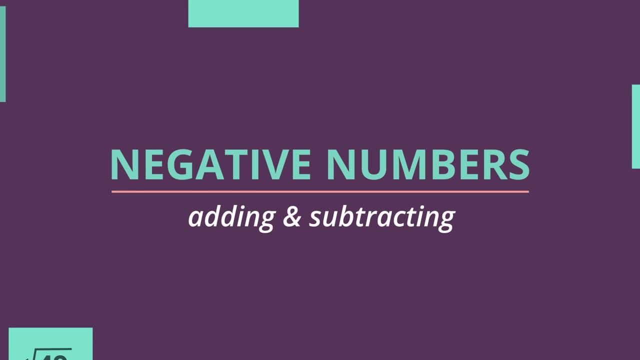 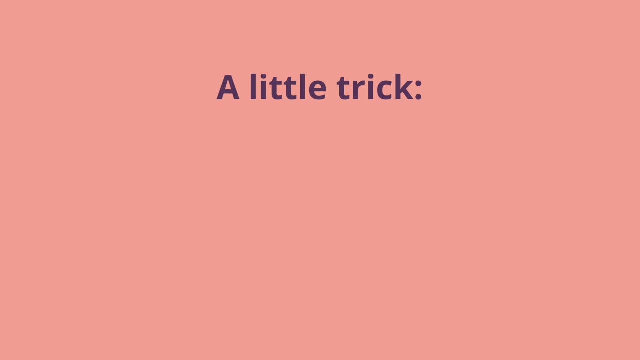 With all of the rules and scenarios. remembering how to add and subtract negative numbers can be difficult. Here's a little trick to help you remember. Let's say we want to solve 3 plus negative 7.. First imagine a number line with a bird sitting on our first number, 3.. 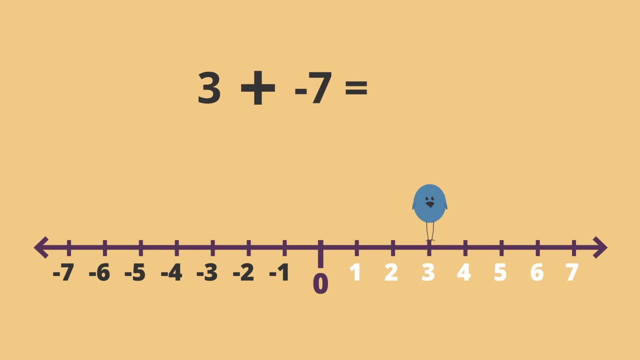 The operation plus or minus tells you which end of the number line to look at. Since we're adding, our little bird will look right towards the positive end. Our second number tells us how far to move and which direction to move. 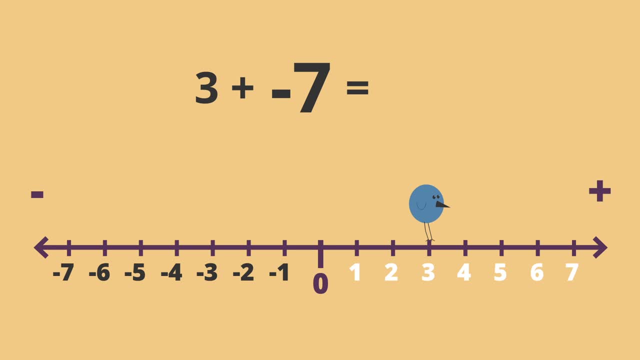 We'll move forward if it's positive and backwards if it's negative. Since our second number is a negative 7, our little bird is going to move backwards 7 spaces Since he landed at negative 4, that's our answer. 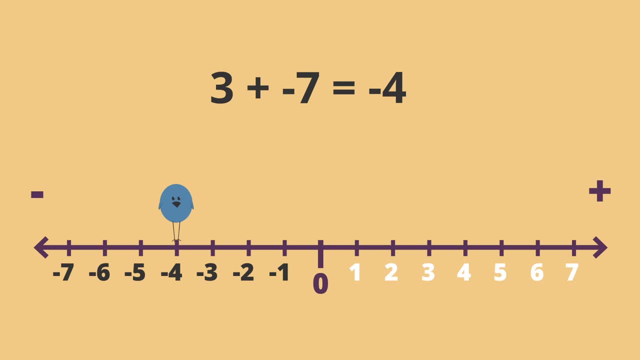 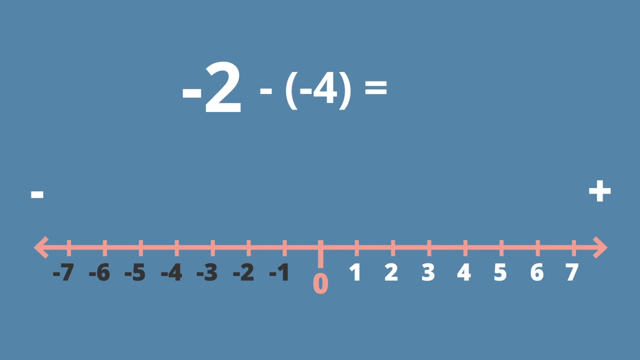 3 plus negative 7 equals negative 4.. Let's try another one. What about negative 2 minus negative 4?? Our first number is negative 2, so that's where we'll start. Our operation is a minus, so our bird will look left towards the negative end. 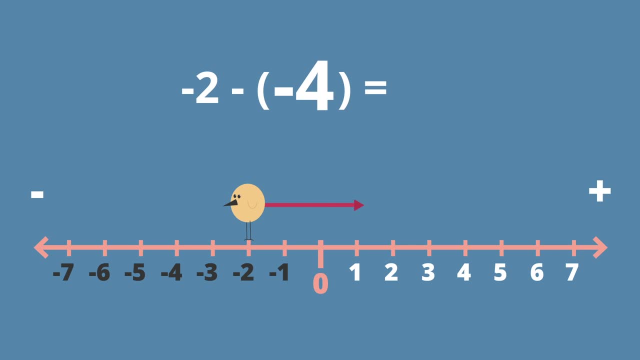 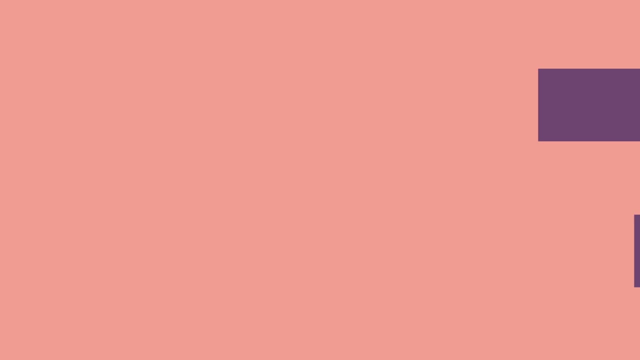 Our second number is a negative 4.. Therefore, our bird will move backwards 4 spaces. Our bird landed at positive 2, and that's our answer. Negative 2 minus negative 4 equals 2.. Let's recap: The first number is where you start. 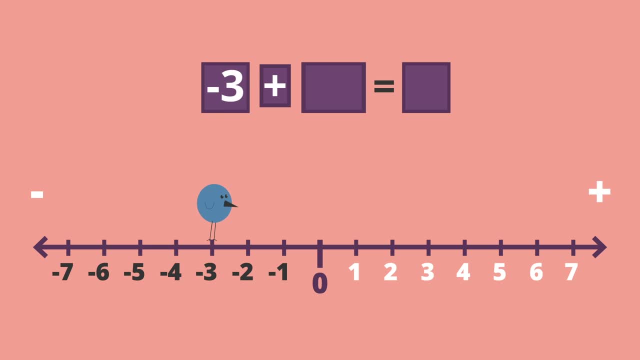 The operation tells you where to look: Plus right or minus left. The second number tells you how far to move and in which direction: Positive forward or negative backwards. Where you land is your answer. That's it. 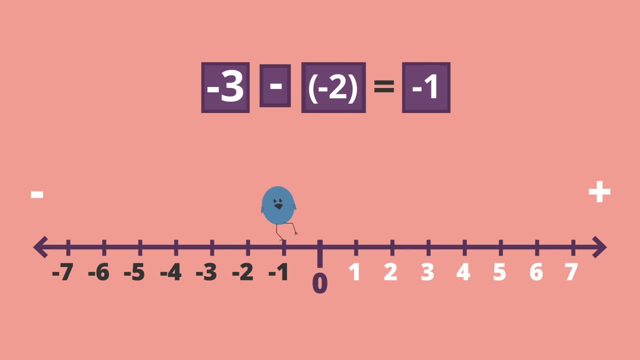 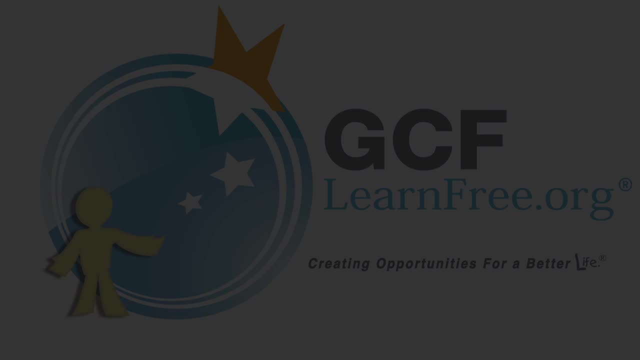 You now know a trick for adding and subtracting negative numbers. That's it. You know the answer. We hope you enjoyed the video. See you later. 3 0 5 1. 1. 1. 2 1 1. 9: 1, 2, 1, 2, 3, 1 2, 1 2 2. 1 1 2.